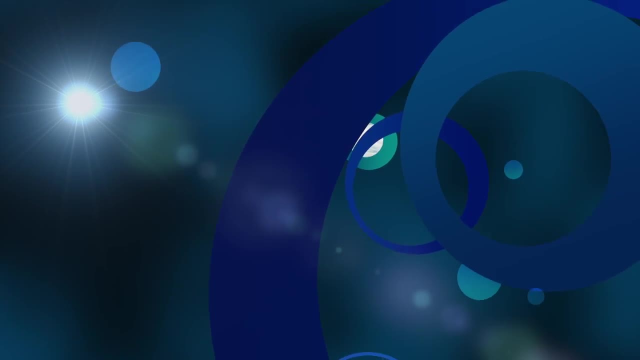 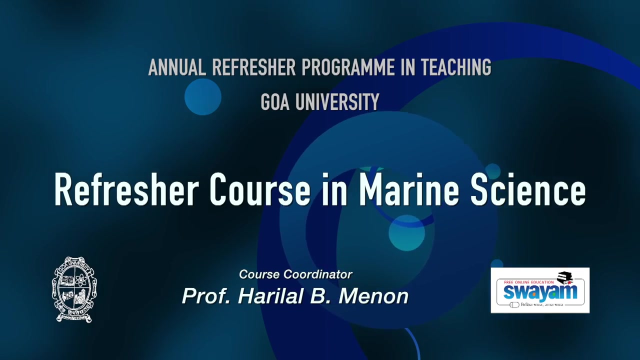 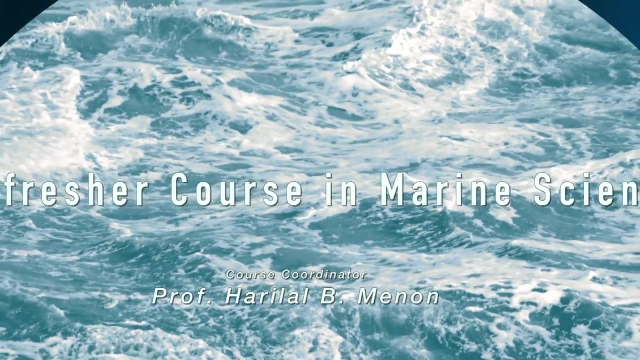 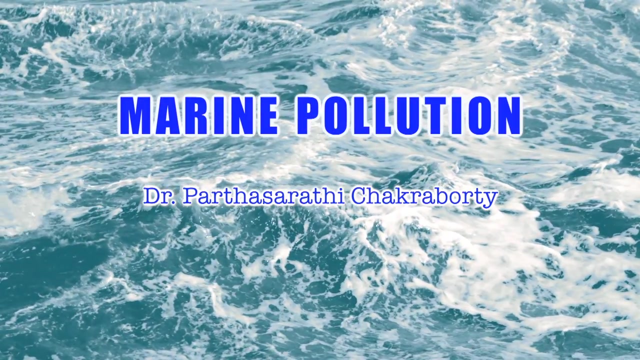 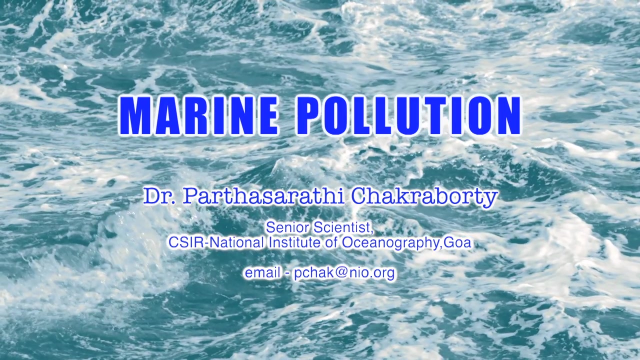 Please subscribe to the channel and press the bell icon to receive notifications when I upload a new video. Thank you very much for watching. Please subscribe to the channel and press the bell icon to receive notifications when I upload a new video. Thank you very much for watching. 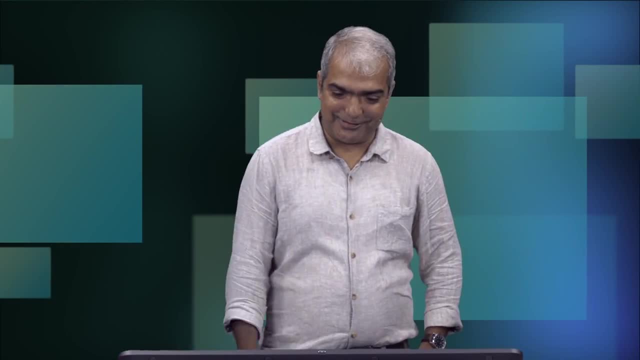 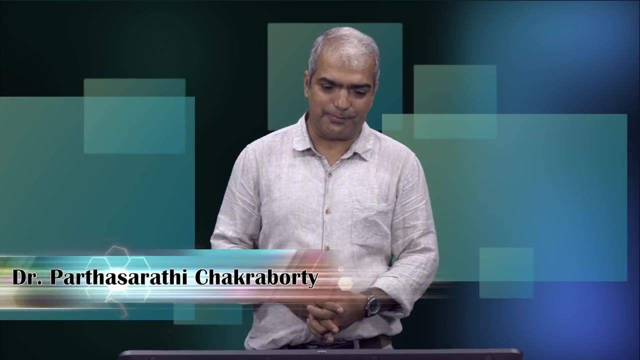 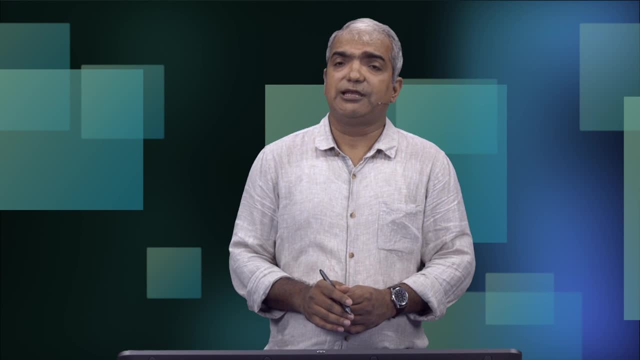 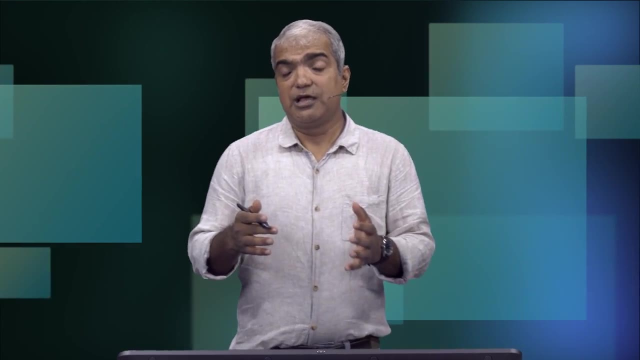 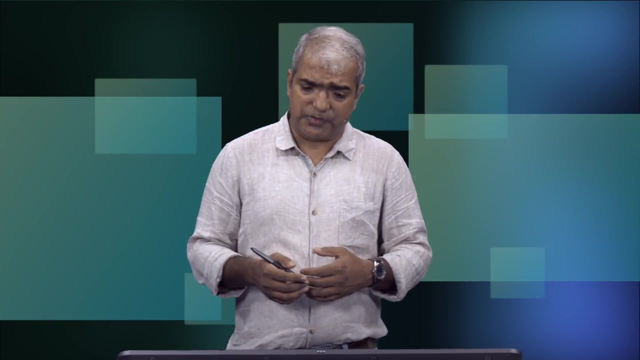 unit is called environment, So basically in an environment where abiotic and biotic both are interacting with each other in a healthy manner. So then it is called a healthy environment. Now what we do: because of human activities we introduce so many different materials. 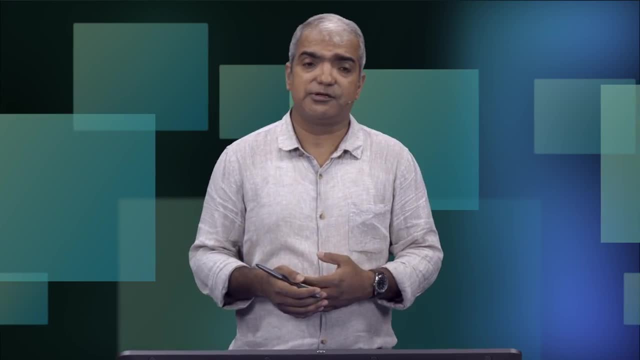 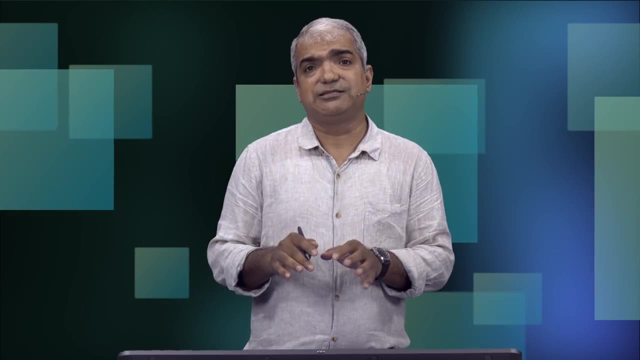 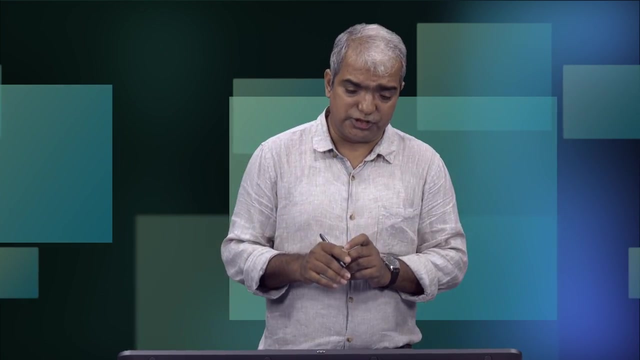 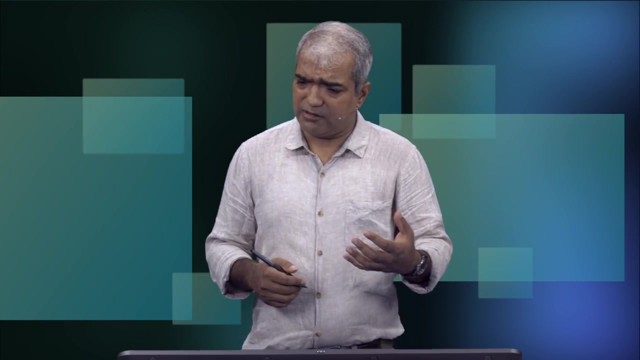 into the environment. We destabilize the material and introduce into the environment and that disbalance that basically changed the delicate balance, altered the delicate balance between biotic and abiotic compartment in the environment and that causes pollution. So you know this is not in India. pollution has been taken very casually till date and everywhere. 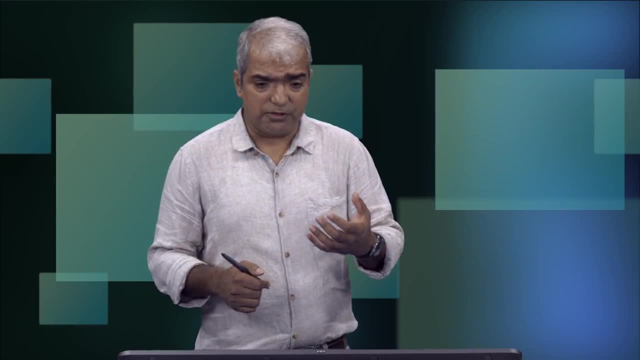 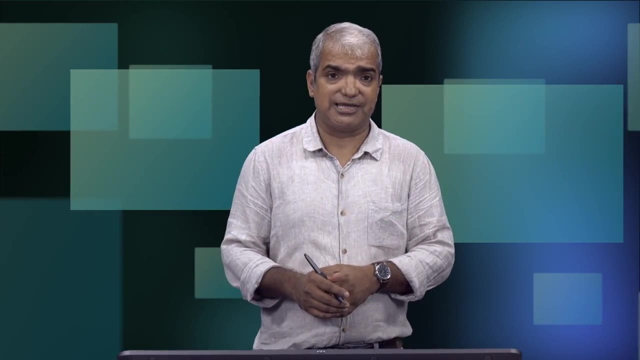 pollution. the subject marine pollution has not been, you know, considered as a very rich science. but it is a very rich science, So we have to take care of it. So we have to take care of it. It has lots of things to understand. You cannot just do it, You know here, first you need to. 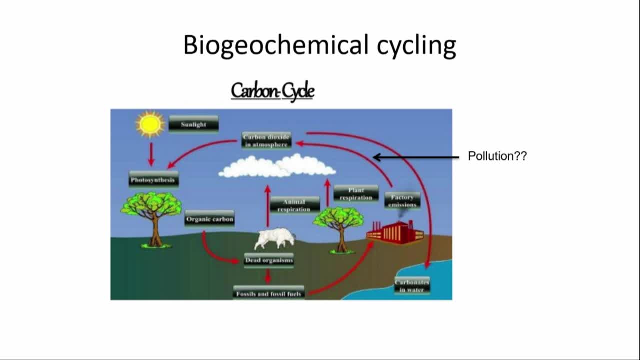 understand biogeochemical cycling. In a healthy environment the biogeochemical cycling takes place where you know. I gave an example here. There are factory that produces lots of carbon dioxide. Plant takes those carbon dioxide here for during photosynthesis and after that the organic carbons. 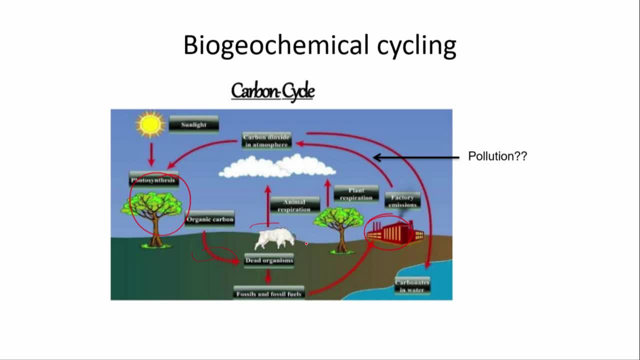 even the vegetations takes place. Then the animal eat those plants and then, after they die, the fossil, the dead organism, becomes fossil and fossil fuels, and a part of that goes to as carbonate in the water and ultimately again they go back to the carbon dioxide. So basically this: this is a simple example of biogeochemical cycling. But now 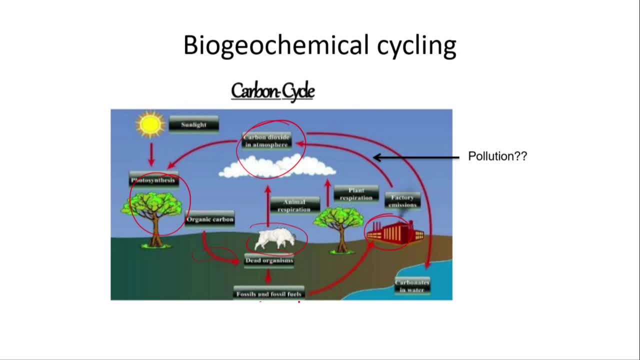 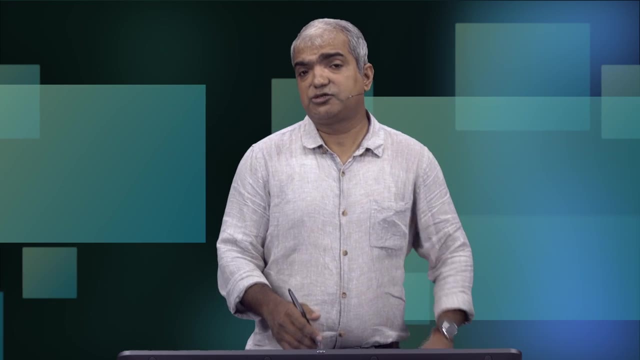 when we take out this fossil fuel from the ground and which were stable, and then use them in factory and produce more carbon dioxide to the atmosphere, then we destabilize the system And that is a kind of pollution that we have been doing it. So this is just an example of carbon There are, so 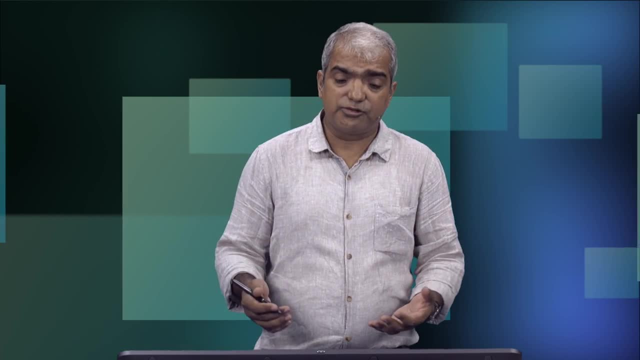 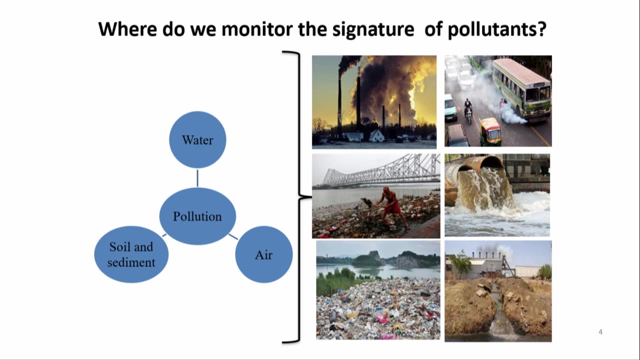 many other materials that we are introducing to the environment every day and that can have catastrophic effect. So that is called pollution. So now, why do we monitor the signature of pollutants? So basically, in water we see the changes in pollutant air and soil and sediment. 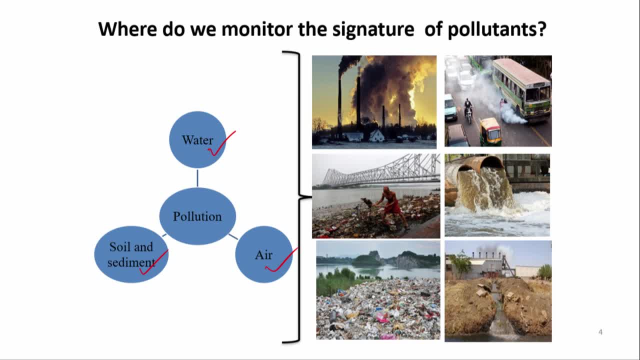 I have shown some examples. like you know, from factories, lots of gases that are going into the atmosphere and remain in the atmosphere, vehicle exhaust, then these are examples of air pollution. then we are releasing lots of effluents into the river or in the coastal environment. 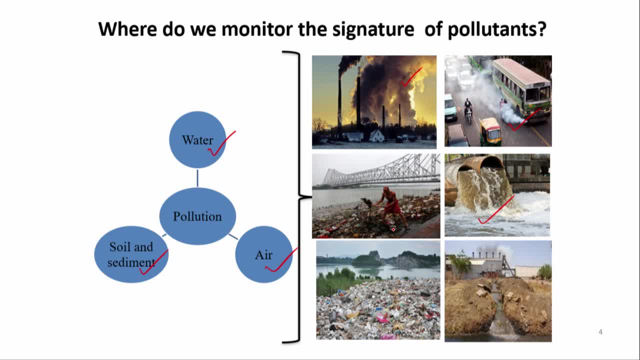 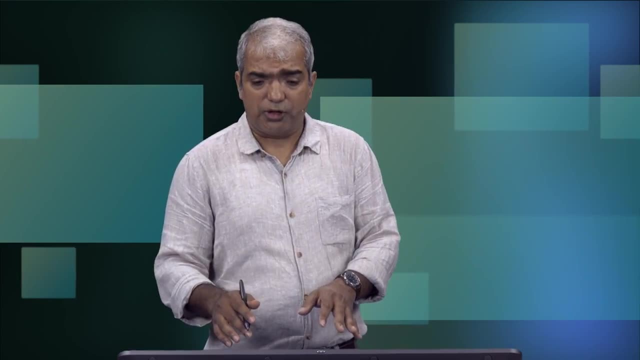 that is water pollution. Then you know we do dump lots of solid waste into the environment, So those are soil pollution. So these are the pollutions that are happening every day. life and that causes, that disbalances or changes the delicate balance between biotic and abiotic system. 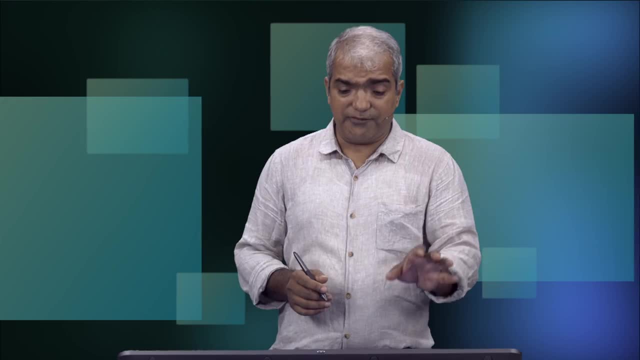 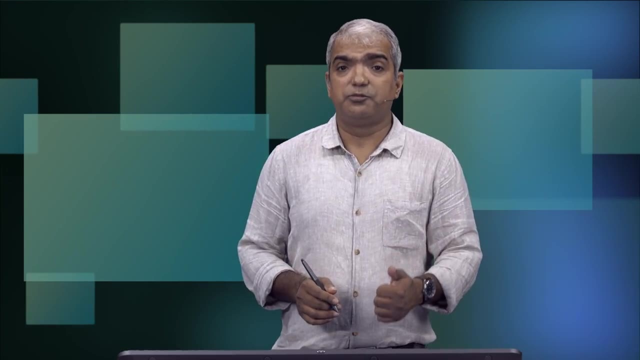 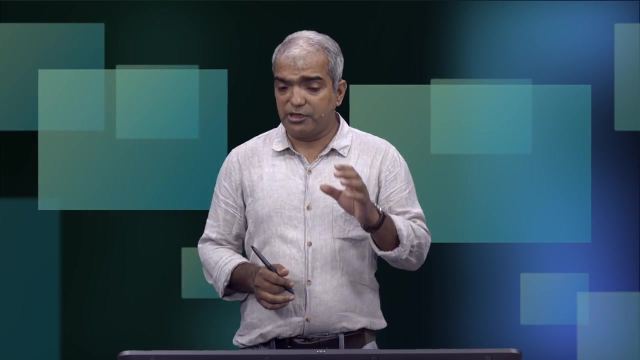 Why should we bother about pollution? Particularly, if you look at particularly in the developing countries, the pollution is a big problem. In developing countries means we have growing economies, we have high rate of industrialization, we have high population In the growing, in the growing country, in the growing. 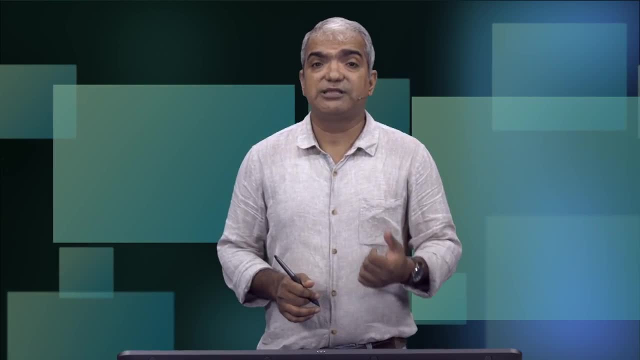 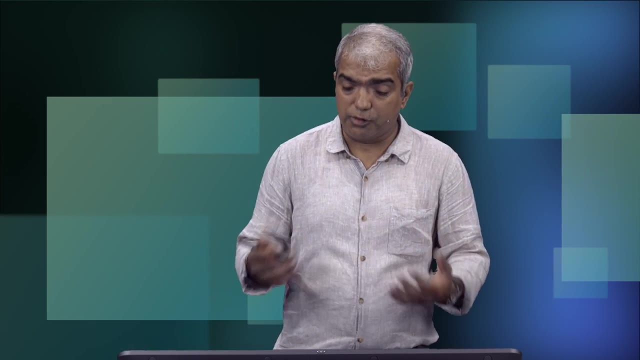 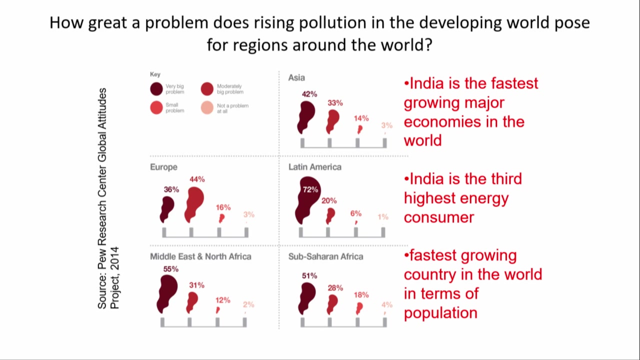 in developing countries. these are all parameters that are growing, So they need more energy And when you need more energy, when there are more industrialization, there will be more pollution And that has been reported And where it shows: in Asia, in Europe, in Latin America, in Middle. 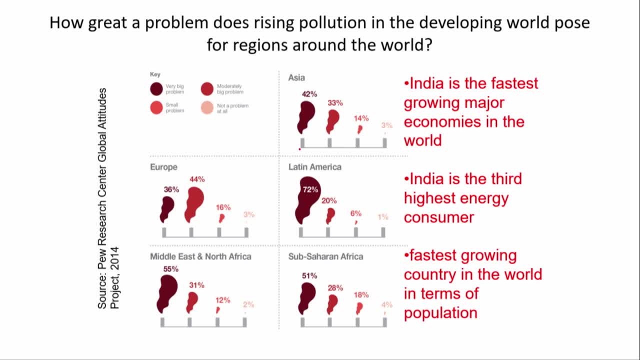 East and North America and Sub-Saharan, everywhere. you know this is a very big problem in almost all the countries, all the developing countries. that developing countries are facing the highest problem because of pollution. India is the fastest growing major economies in the world. 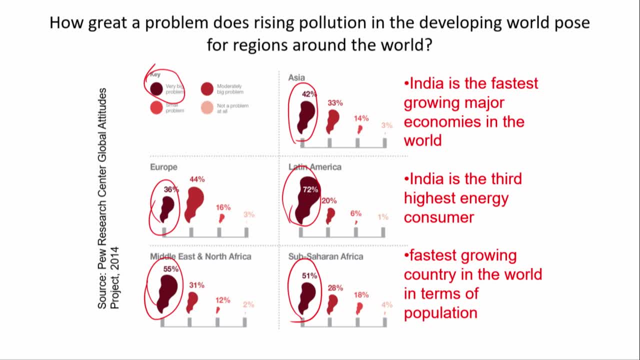 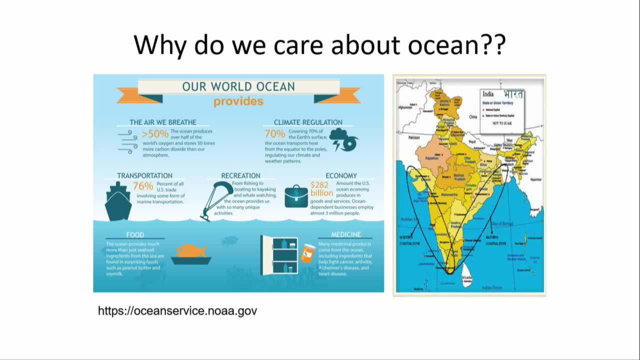 India is the third highest energy consumer and, you know, fastest growing country in terms of population. So we must care about pollution on land. But why should we worry about ocean when we live on land? It is because, you know, the ocean produces almost half of 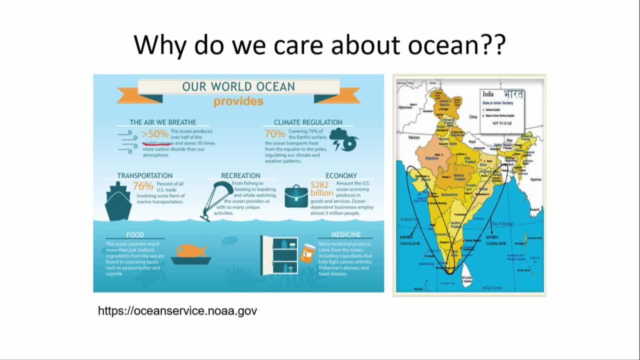 the world. oxygen And 50 times more carbon dioxide are present are stored in ocean compared to the atmosphere, So it is an important place where we get lots of oxygen for our expression. Secondly, it regulates climate. It regulates climate And because monsoon, starting from. 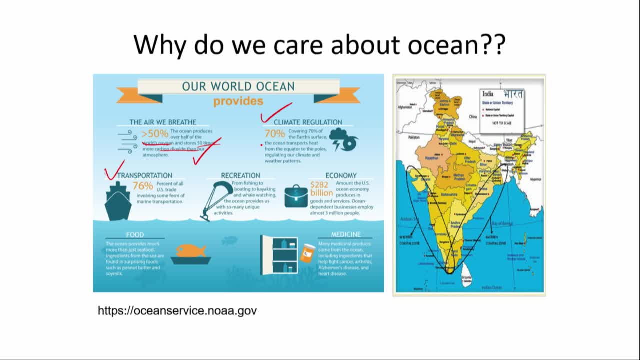 monsoon and drought, all these things are regulated. And then it regulates the climate And because monsoon, starting from monsoon, and drought, all these things are regulated by the ocean and ocean temperature. We get lots of seafood and medicine from the ocean. 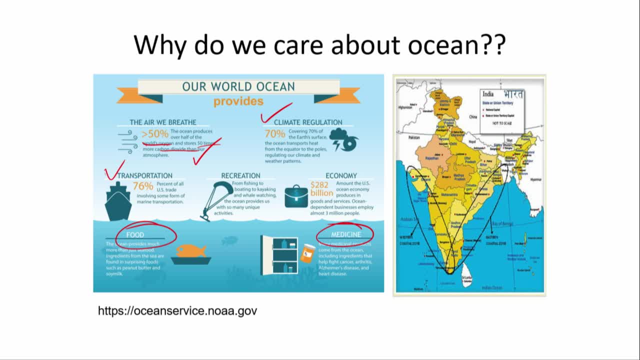 So we must take care of it. If you look at India's map, we have a coastline of 7,500 km. We get a huge amount of resources from this area, So we need to take care of this area. Whatever we do on land affects coastal areas. 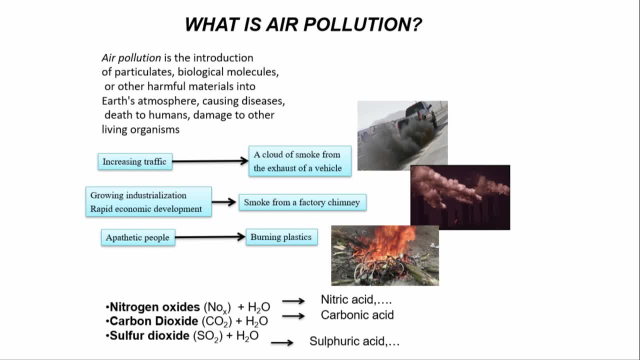 So we must know about the different types of pollution. You must have heard of air pollution, where we introduce pollutants into the atmosphere. We produce lots of traffic increases, smoke from the exhaust, carbon dioxide, carbon monoxide, sulfur dioxide, nitrogen dioxide. 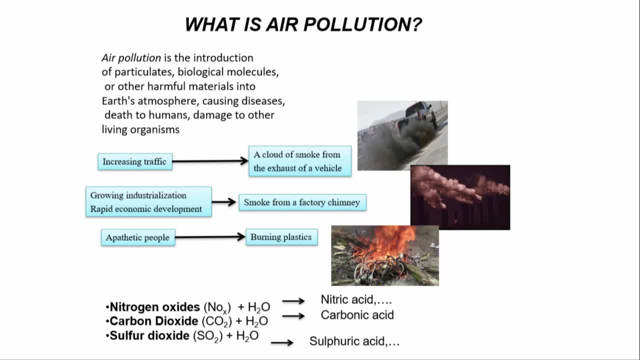 We also burn lots of plastics and all these different types of unwanted materials into the environment, and that produces lots of gas. Now what happens to these gases? These gases go to the atmosphere, it combines with water and it forms strong acids like nitric acid. 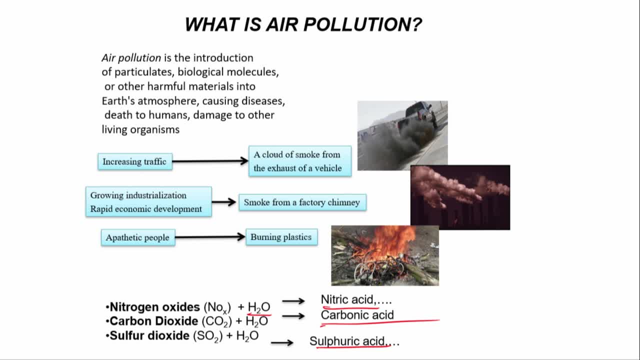 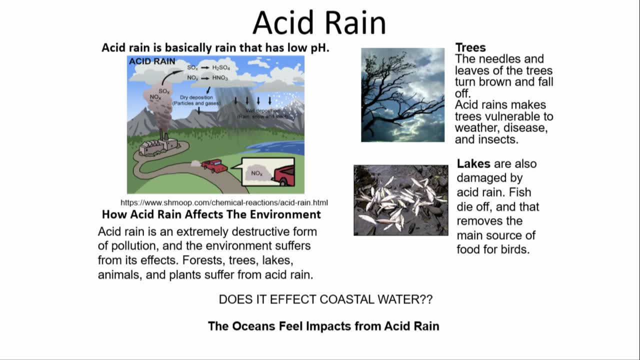 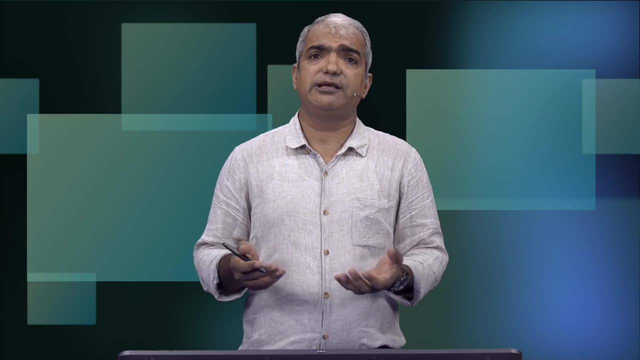 sulfuric acid, even weak acids like carbon dioxide. So these are the things that happen on land Because of atmospheric pollution. the gas goes to the atmosphere and they combine with water and then form acids. It can be strong acid, it can be weak acid, like nitric acid, sulfuric acid. These are strong acids and carbonic acid is a weak acid. So whatever the gas is like sulfur dioxide, nitrogen dioxide or carbon dioxide- it can go to the atmosphere, it combines with the moisture, it can form acid and it can come back to the land with rain. 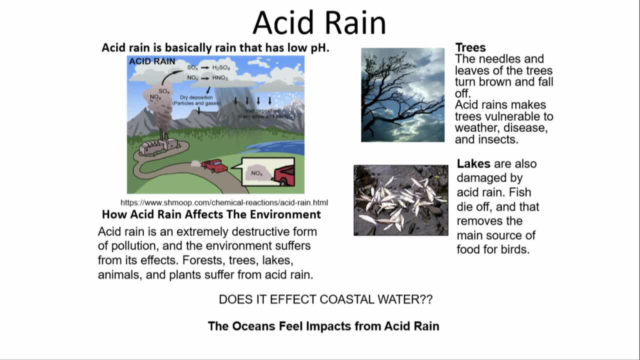 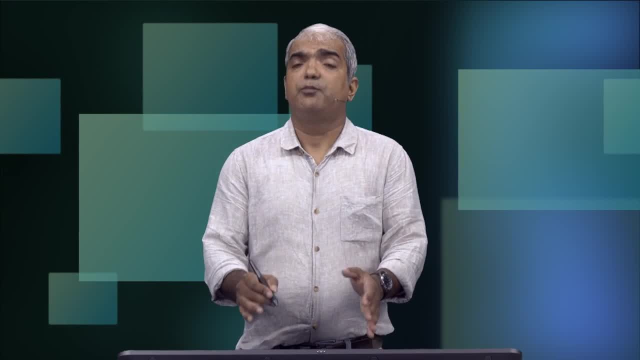 At that time it is called acid rain, and this acid rain can be detrimental to the living organism in a particular area. Now this is happening in land, but this rain can be precipitated even in the coastal water, where it can have impact. 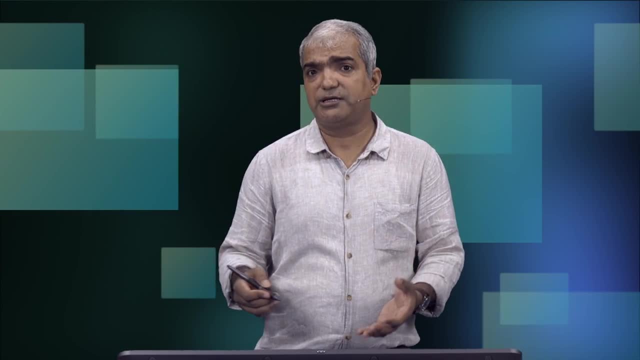 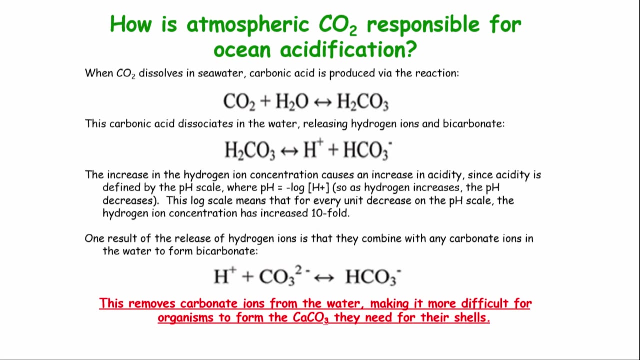 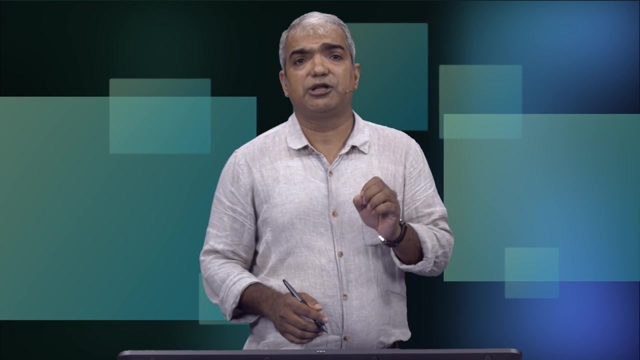 on the marine ecosystem. It can affect phytoplankton, it can affect fish. So that has been found. But what about the open ocean If you go far away from the coastal areas? there, the most important gas that affects is carbon dioxide, not sulfuric acid or sulfur dioxide. 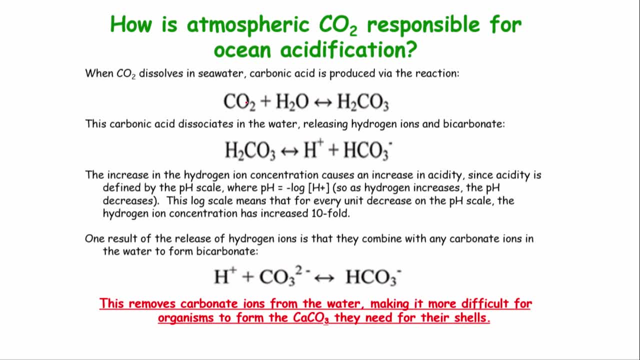 or nitrogen dioxide. Here we know that carbon dioxide, when it interacts, when it reacts with water, it forms carbonic acid and this carbonic acid dissociates to protons and bicarbonate ions And you know this proton. basically, when carbon dioxide 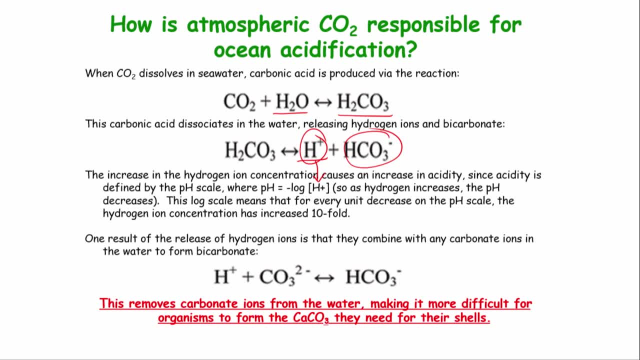 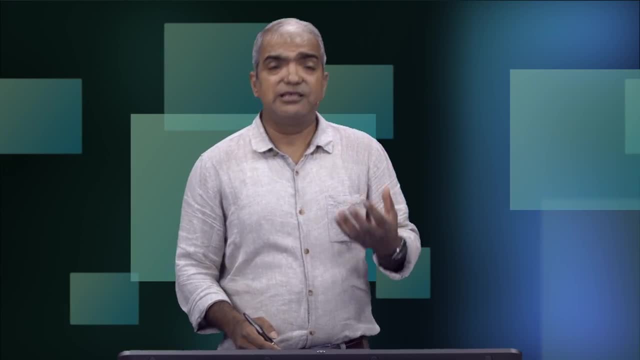 gets dissolved on the surface water- surface ocean water- it forms carbonic acid and then this carbonic acid dissociates to protons and bicarbonate And this proton basically decreases the pH of the ocean- surface ocean- And this is called ocean acidification And this ocean acidification can cause tremendous 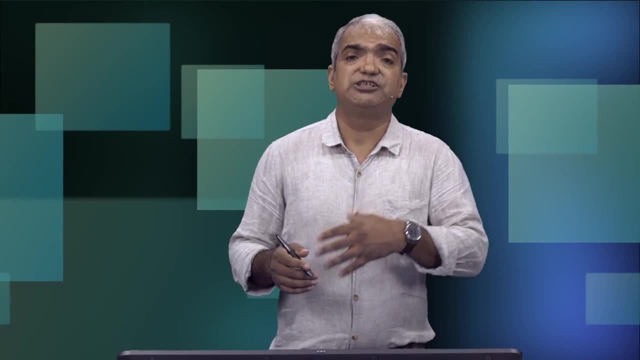 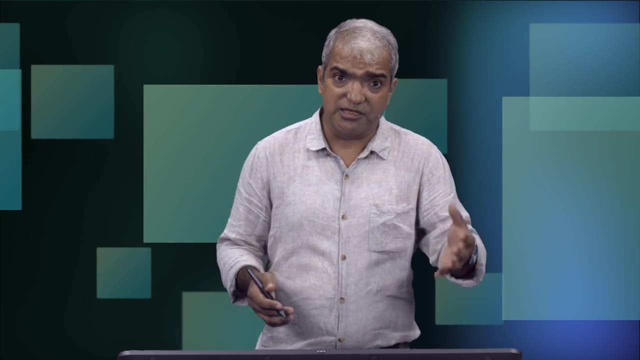 problems on the phytoplankton community as well, as it can change the fisheries and it can change, you know, the other pollution such as you know, indirectly, by lowering the pH, it can change the mobility, bioavailability of different. 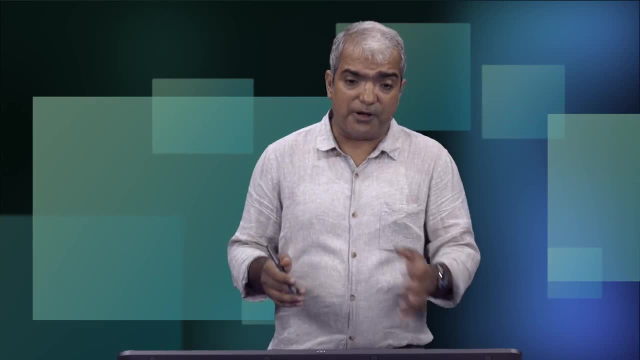 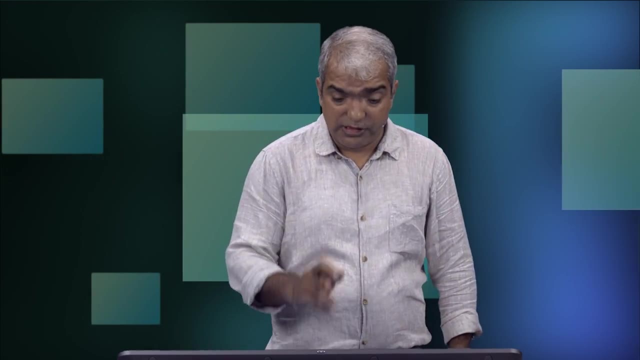 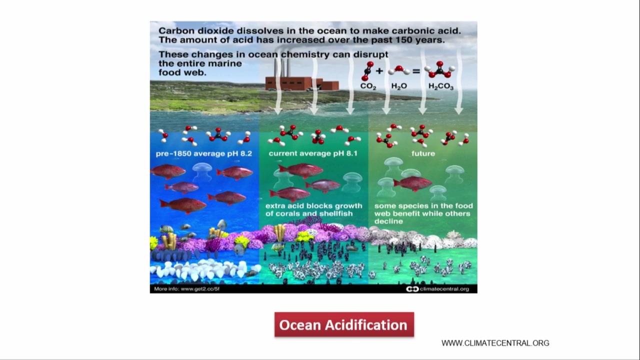 toxic species, toxic metals, toxic compounds in marine environment. So carbon dioxide we are producing on land, but it is affecting open ocean, So we should care about air pollution. Now here I showed one example. You know, pre-industrialized. 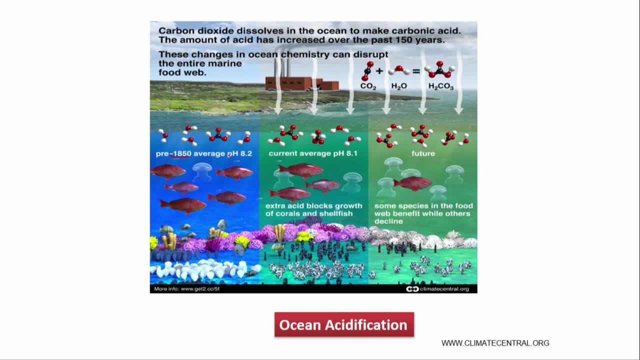 before industrialization started in 1850, the average pH was 8.2, and current average is 8.2,. but in future, if we keep producing carbon dioxide in this rate, then probably it will go further down and that can have tremendous. 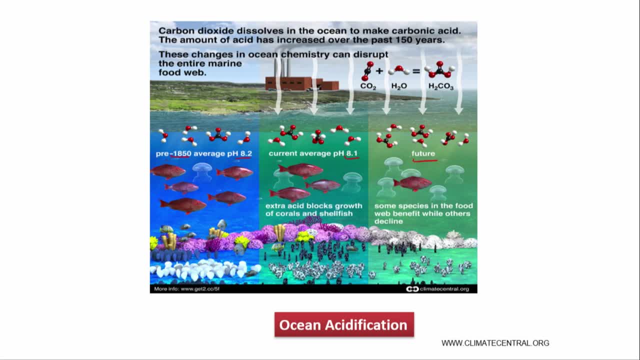 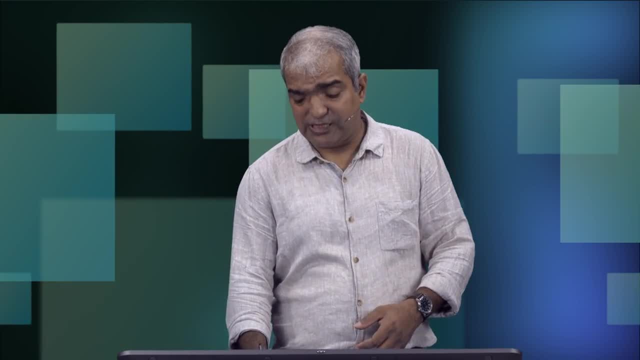 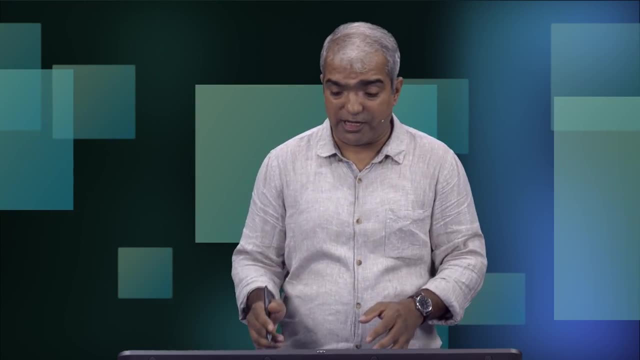 impact on the corals like, or the organisms which are having calcium carbonate kind of shell. It can dissolve those calcium carbonate and, you know, those species will die and biodiversity of marine system probably will be destroyed. So it's a very delicate system. 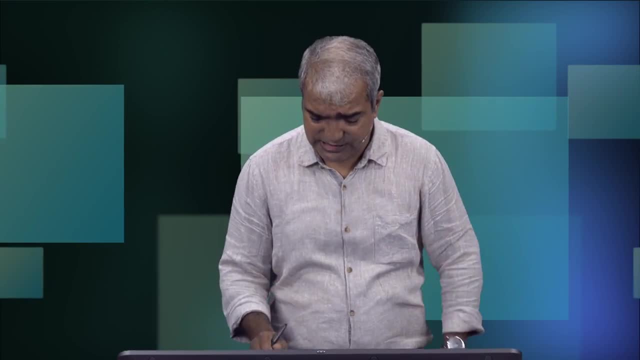 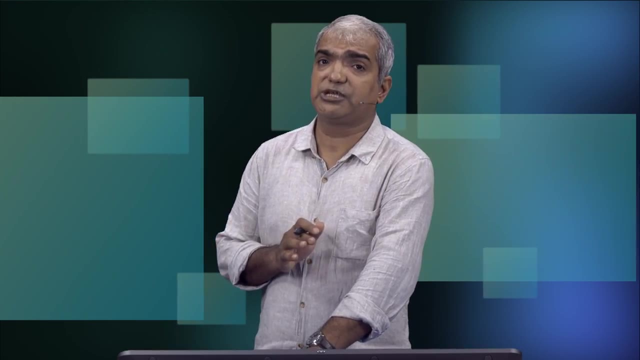 So whatever we do on land, that can have impact in the marine system. So this process is called ocean acidification. So this is just an example I'm giving that atmospheric pollution can cause tremendous problem even in open ocean. Now, 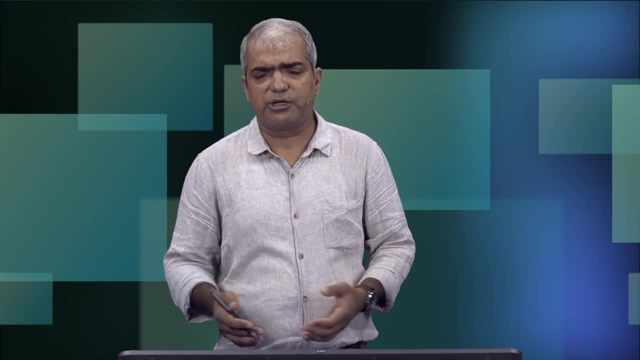 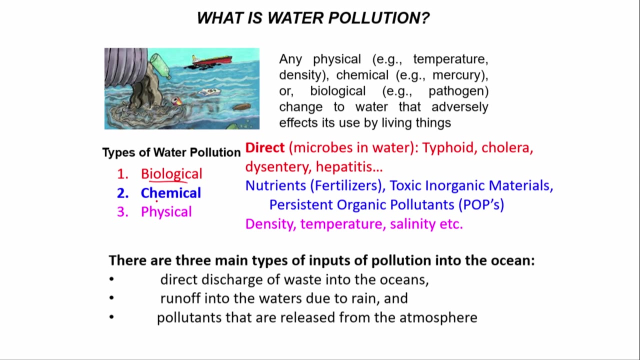 water pollution. So water pollution, there are different types of water pollution, happens every day in our daily life. So but I'm going to. it can be biological, it can be chemical, it can be physical. In chemicals, you know, nutrient, toxic, inorganic materials, persistent, organic. 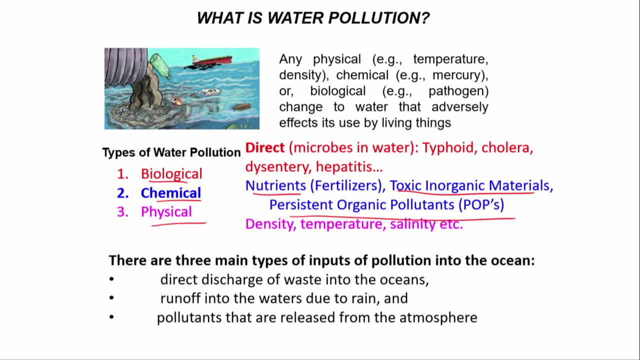 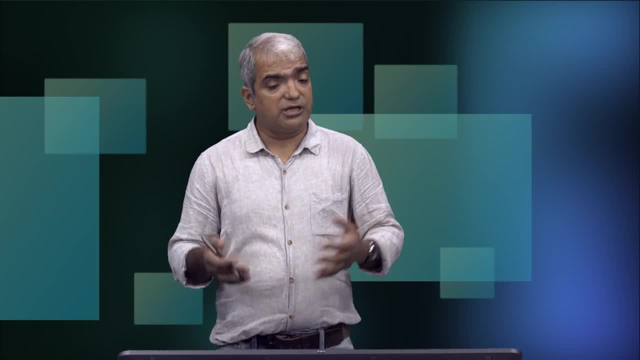 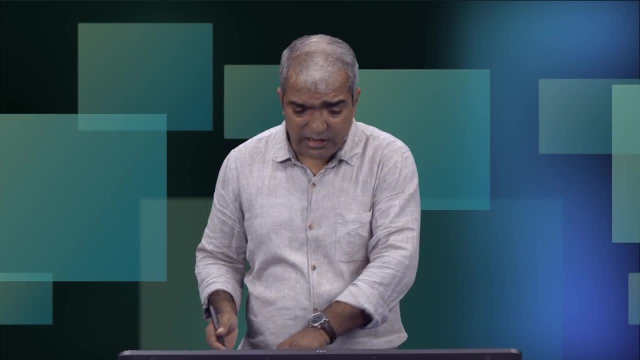 pollutants. these are the major chemicals that every day get released into our environment and ultimately it get sink into the coastal water or in a seawater. So what are the impacts of those That also we don't know? Now you know, if you see here eutrophication. 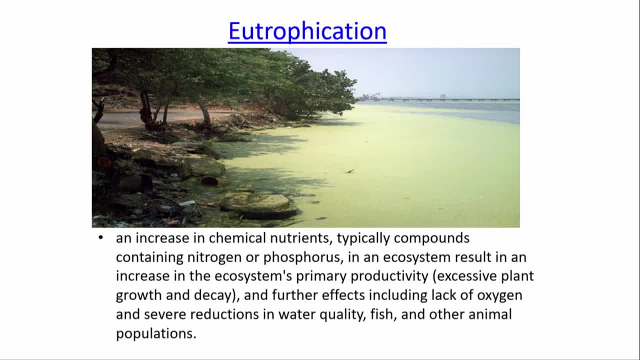 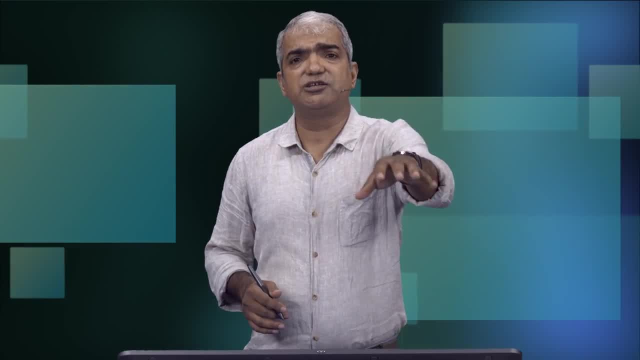 we have a long coastline, we have agricultural field. during land runoff, lots of nutrient, you know, washed off from the agricultural field and it goes into and get discharged into the coastal water And these nutrients are rich in nitrogen and phosphorus, which helps. 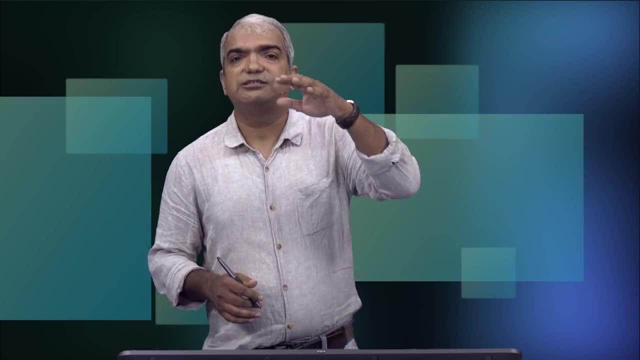 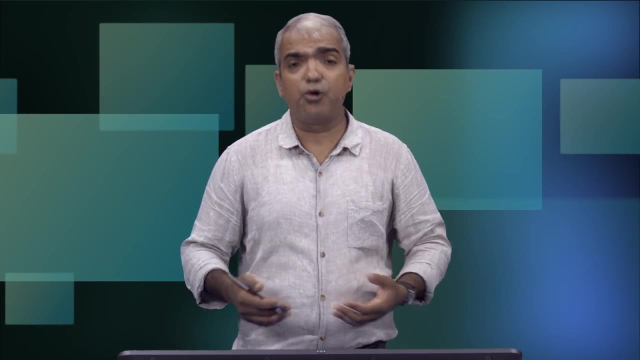 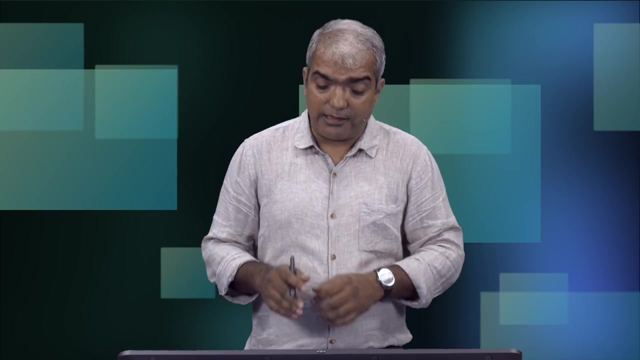 the phytoplankton, the small, tiny plants on the surface of ocean. they use them as a nutrient and you know they grow in a very fast rate and that causes that known known as. that is known as bloom, and 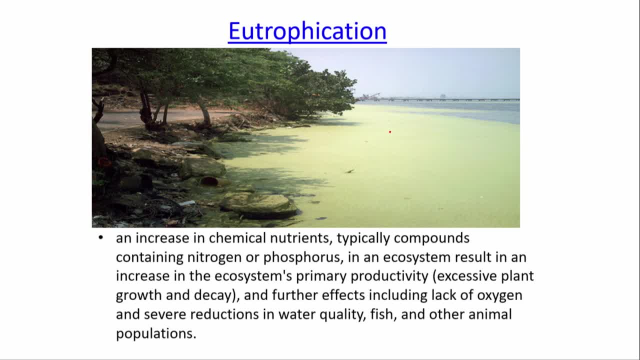 those such kind of phytoplankton bloom takes place. Now, here I have shown. have you seen that green color, the green patches? this is called phytoplankton bloom because of supply of nutrient, more nutrient, lots of phytoplankton. 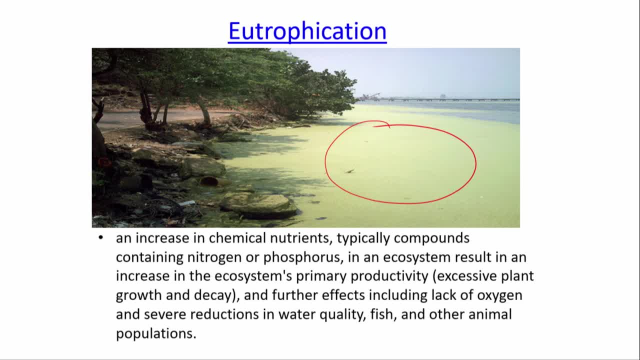 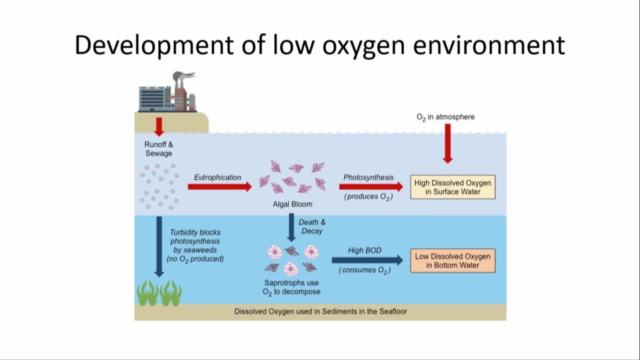 grow and they form a layer on the top of the surface ocean. Now, if the surface ocean get covered with this green bloom, then what happens? You know basically what happens. the ox, the surface layer, a particular layer. it. 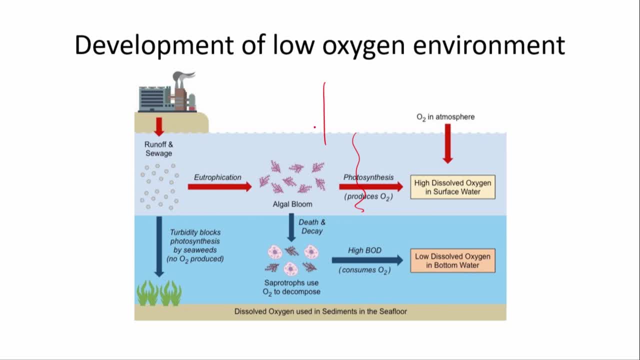 produces oxygen but at the same time it prevents any oxygen to go in further down. It stops oxygen to go in, go down further and as a result the oxygen concentration here decreases drastically. And when it decreases drastically, this oxygen, this area, this 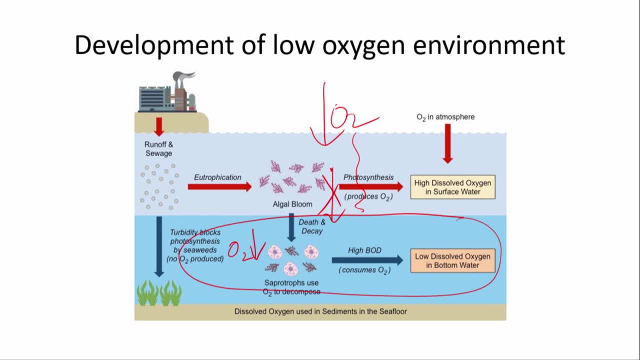 whole area become low oxygen. low develop a low oxygen environment and with time, if this bloom remain for a long time then oxygen cannot penetrate for long and at the same time this lower part become much lower in oxygen and then it become a dead zone. 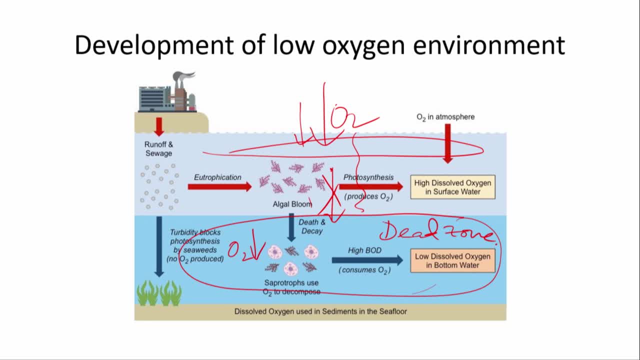 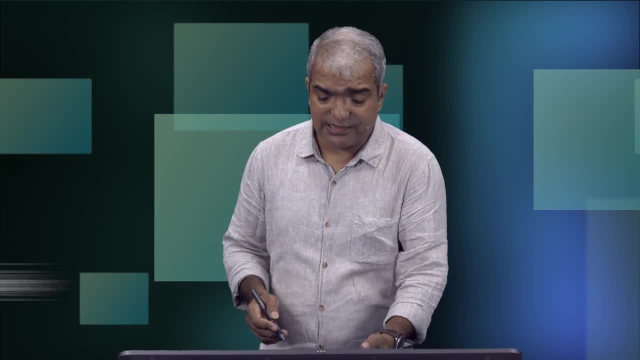 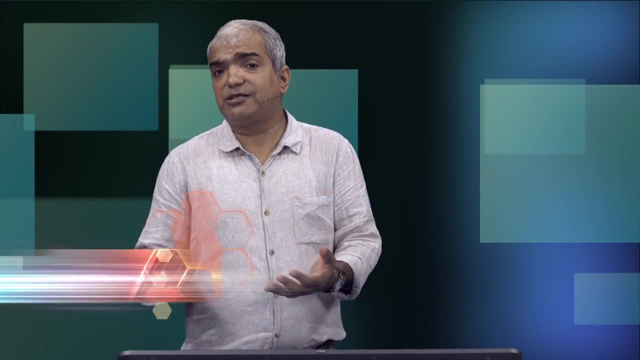 And when it become a dead zone then you must understand, in this low oxygen environment any commercially like fish, they cannot stay, they move away from this. so it affects the fisheries. So we do our agricultural activity and use of. you know. 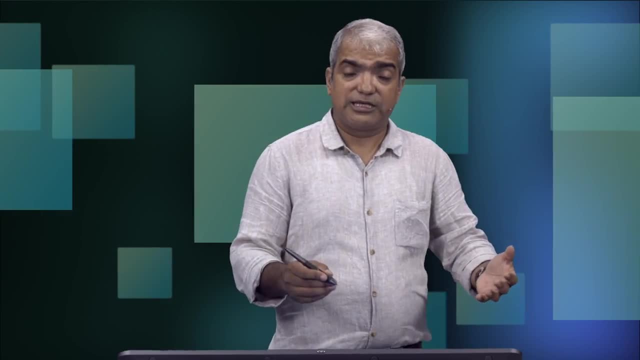 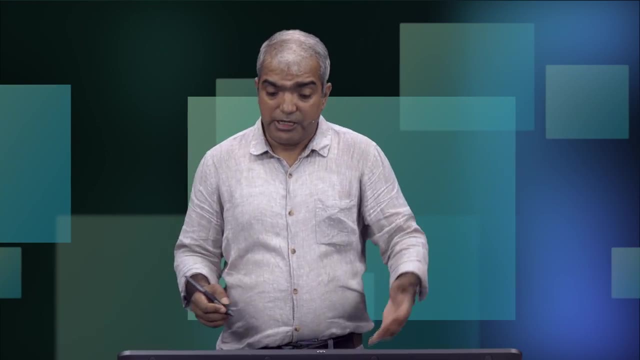 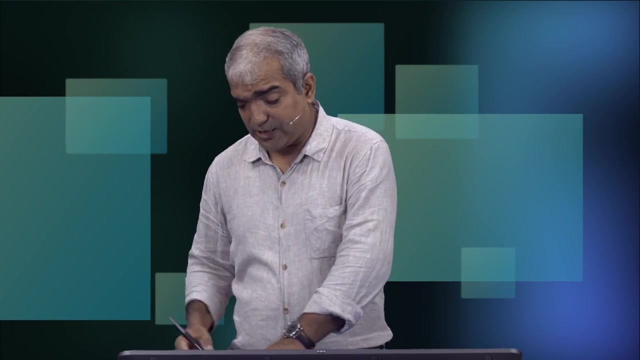 nutrients or fertilizer can have impact- impact on the coastal water and that can have impact on the fisheries, which can affect our economy. So this is very important thing to understand, that you know: whatever we do on land, it can have impact on the coastal. 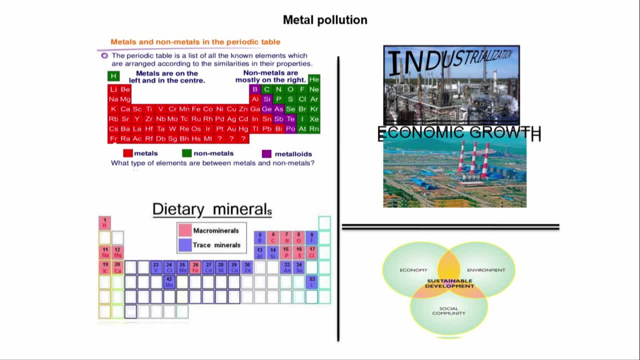 environment. Then come metal pollution. You know this is the periodic table. you must be familiar with this periodic table. you know there are so many elements. The red color, the red color elements are called metals. They are alkali metals, alkaline earth metals, trace metals. 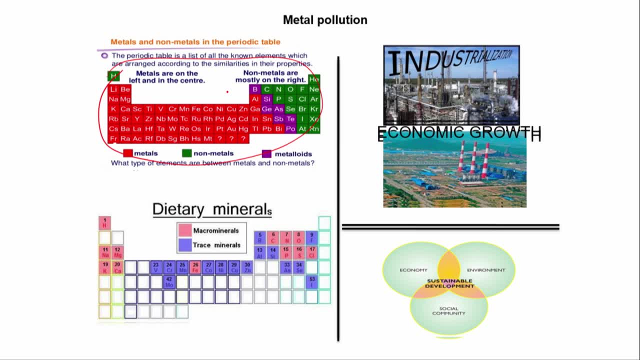 transition metals. So these metals, all these metals, we don't need it for our body. We need some of them as a nutrient, but not all. You know, what we need are these elements that we have shown here. So these elements, 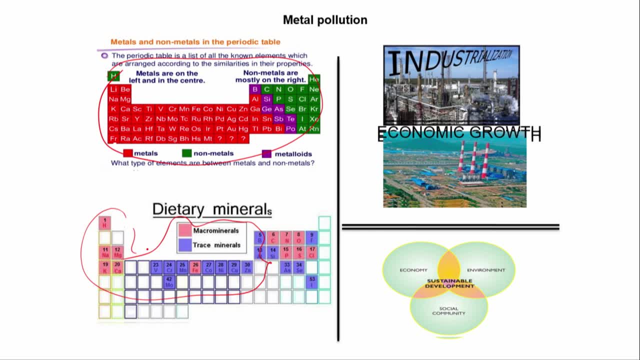 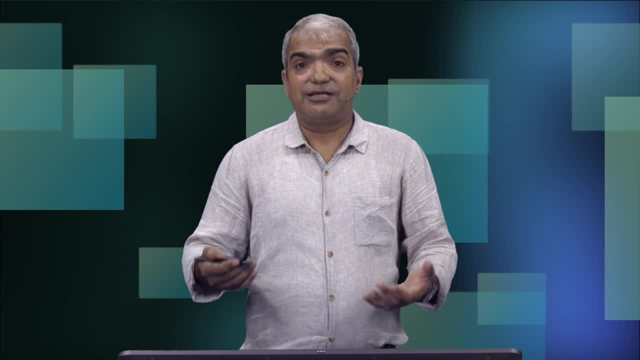 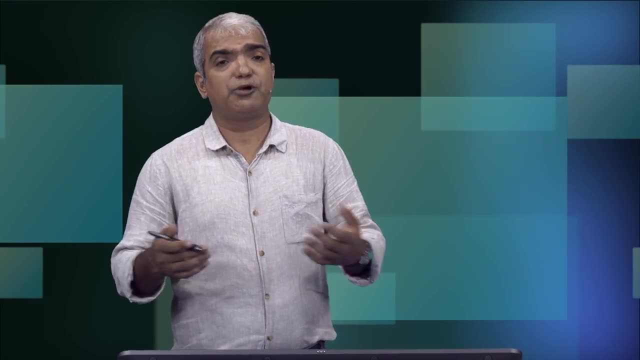 only these elements we require for our existence. but what about the rest of the metals that are present in the periodic table? Those are also required, very much required for our industries. They are used as catalysts, they are used as raw materials for different, for the production of different kind of materials. So 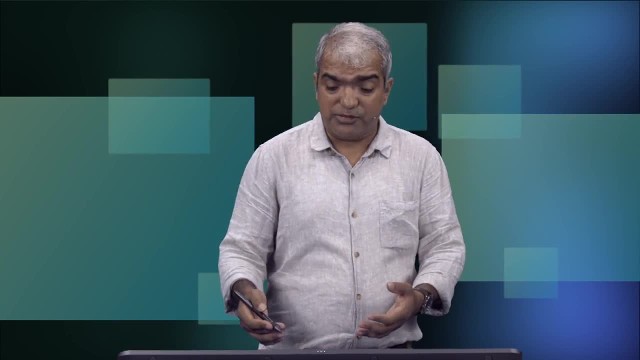 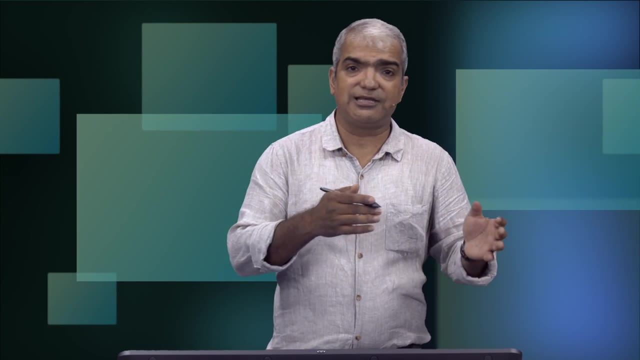 we need industrialization. but at the same time, after you means after their use- we are dumping them either into a coastal environment or on land and from there land runoff takes place and then ultimately it settles in the marine environment. So basically we also get exposed to those. 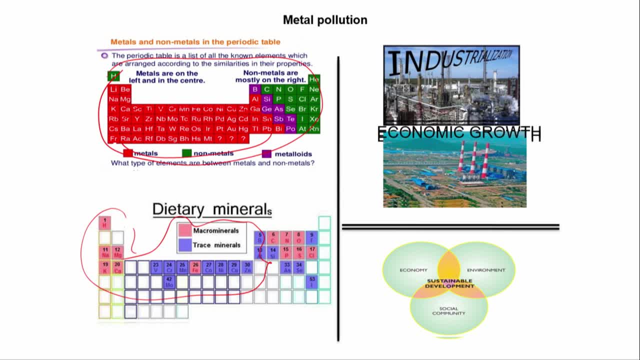 metals which are not required for our body and we get, you know, contaminated by these metals. So what we need to do, we need to have economic growth, we need to have industrialization, but at the same time, we need 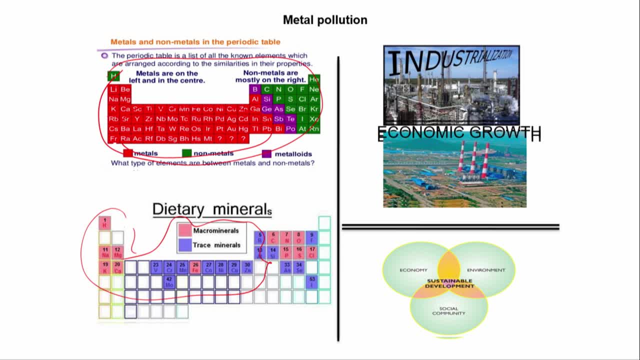 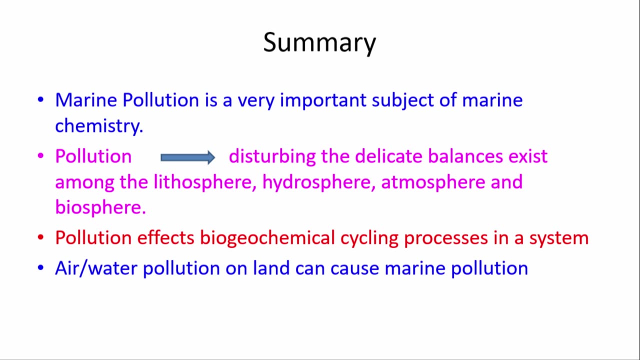 to have sustainable development, We should not do pollution, metal pollution, which can affect our coastal environment, our marine environment as well as our health. So there has to be a balance. So here in the first module, I discuss about marine. 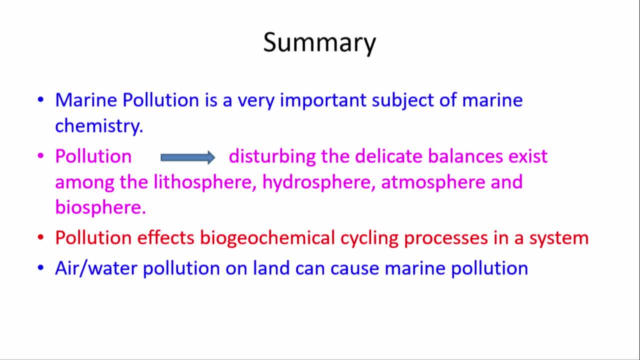 pollution, which is a very important subject and a part of marine chemistry, and pollution is nothing but disturbing. the delicate balance exist among the lithosphere, hydrosphere, atmosphere and biosphere and you know pollution can basically affect the biogeochemical cycling processes in a system. 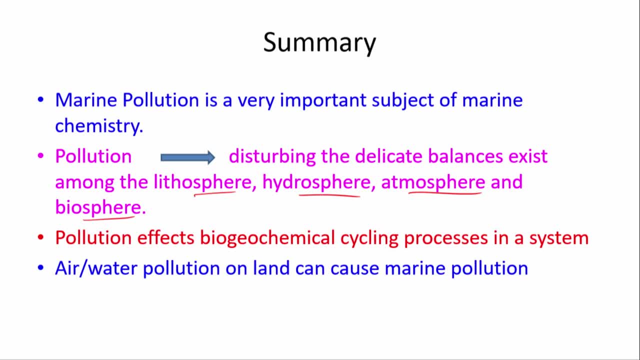 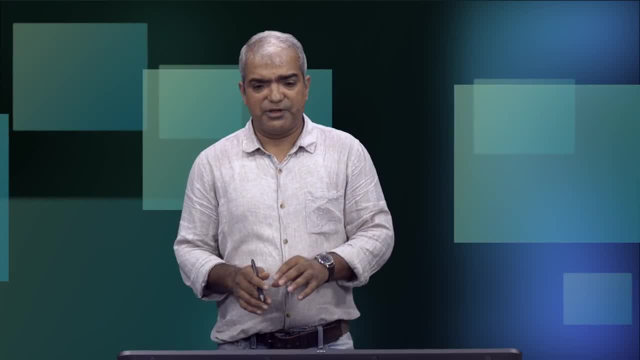 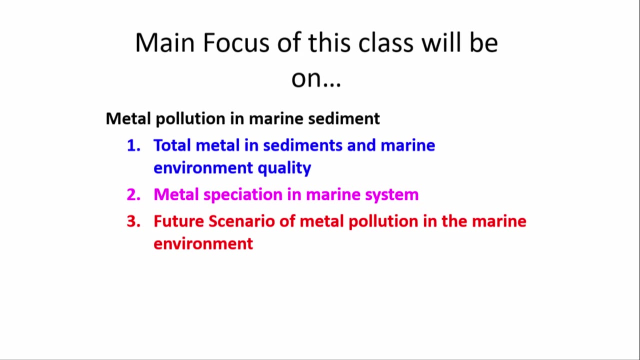 and air-water pollution on land can cause marine pollution. So in this module I discuss about different types of pollution briefly, because here it is not possible to discuss almost all the things in detail. So in the next module I'll be basically talking about the. 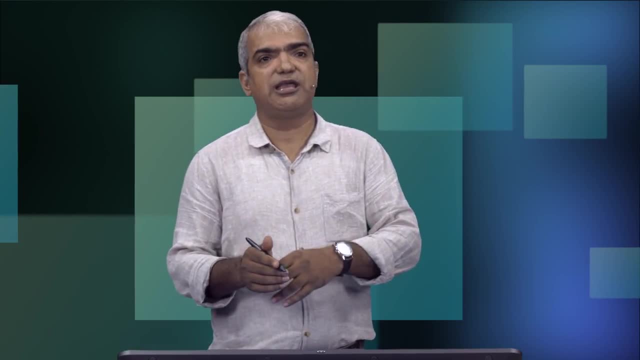 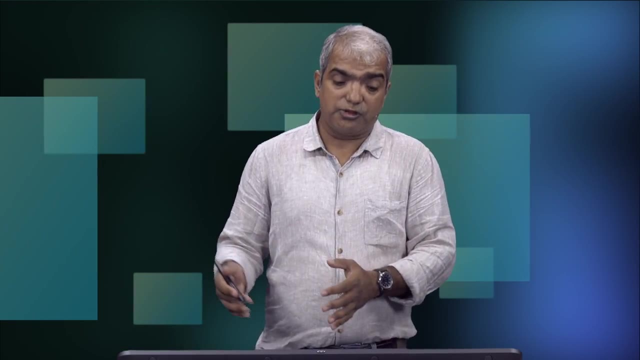 metal pollution in sediments, because pollution can be in any compartment: It can be in lithosphere, it can be in biosphere, it can be in hydrosphere. but in the next module I'll talk about metal pollution in marine sediments and